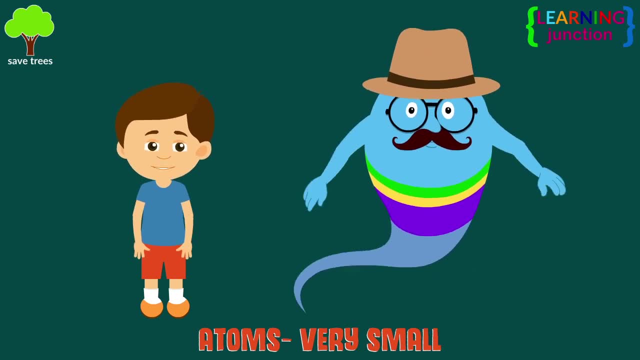 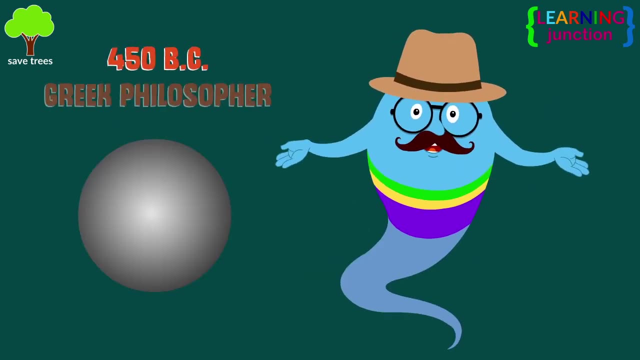 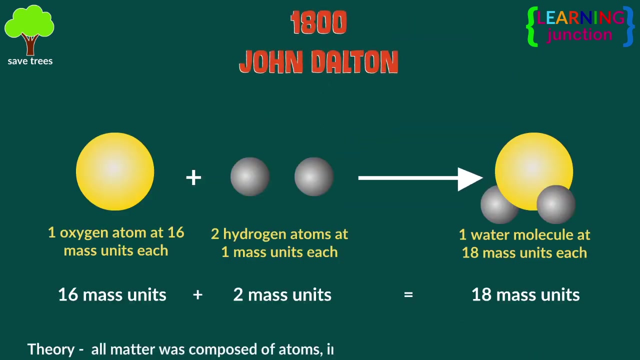 Atoms are so small that we cannot see them. Even the most powerful microscopes can't visualize single atoms. Around 450 BC, Greek philosopher Democritus introduced the concept of the atom. In 1800, John Dalton reintroduced the atom. 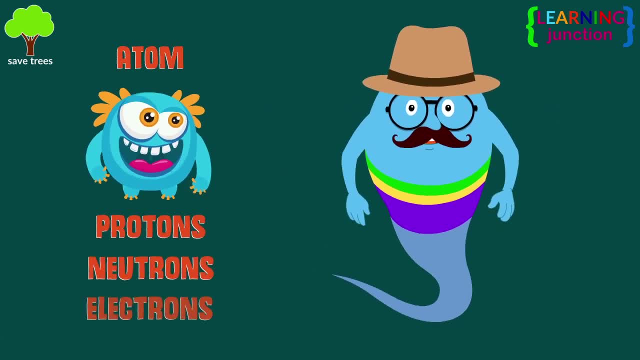 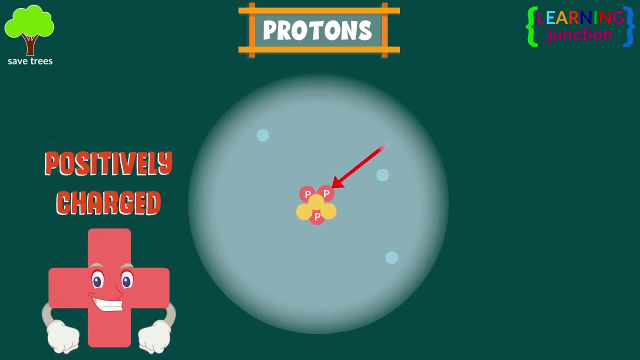 An atom is made up of three parts: protons, neutrons and electrons. Come on, let's learn about these one by one. Protons: A proton is a positively charged particle found in the atmosphere. It is held within the nucleus of an atom. 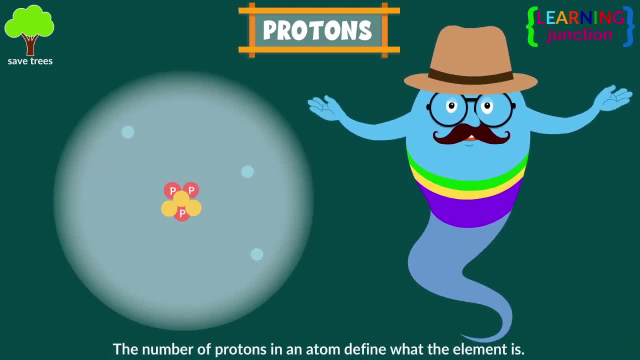 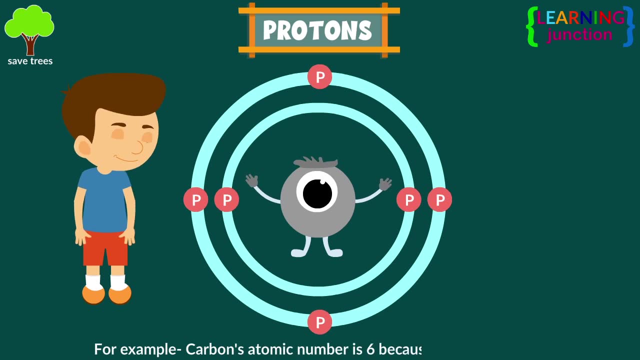 The number of protons in an atom define what the element is. This is referred to as the atomic number of that element. For example, carbon's atomic number is 6 because it has 6 protons. The number of protons also determines the chemical properties of an element. 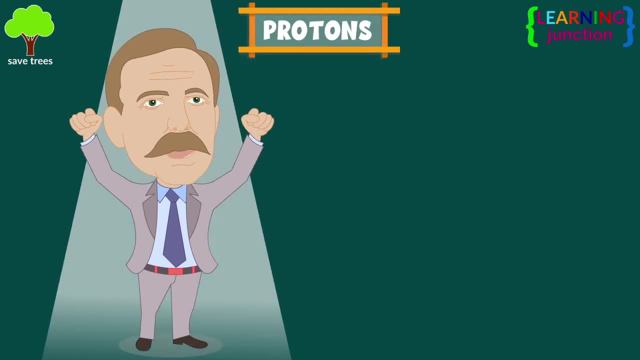 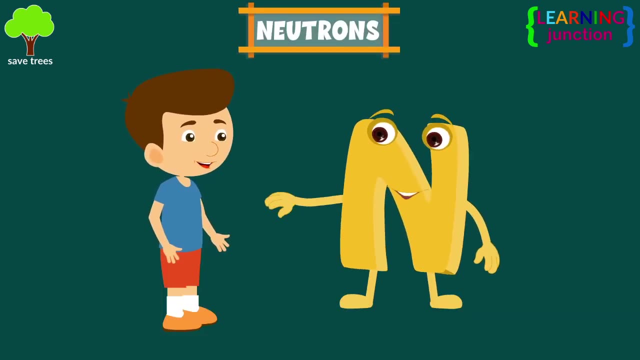 Protons were discovered by a New Zealand-based physicist, Ernest Rutherford, in the early 1900s. And now let's learn about the atom, Now the neutrons. Let's have a look. A neutron is the neutral part of the nucleus of an atom. 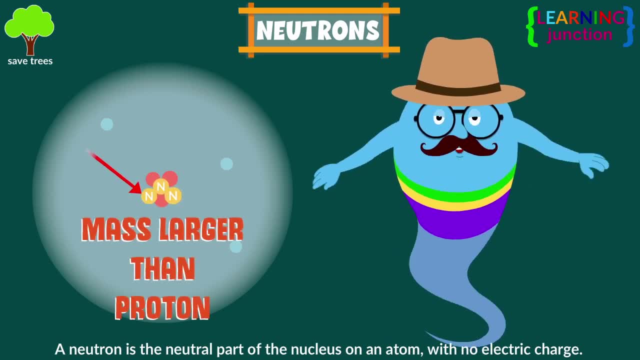 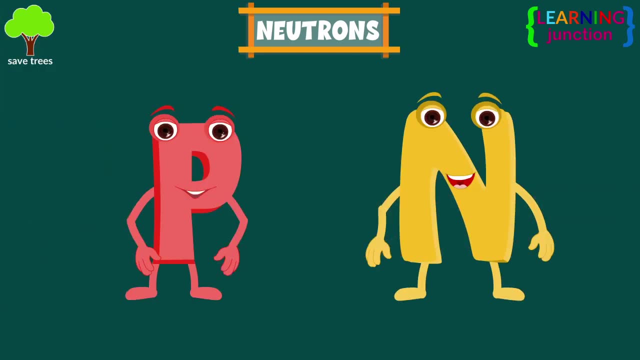 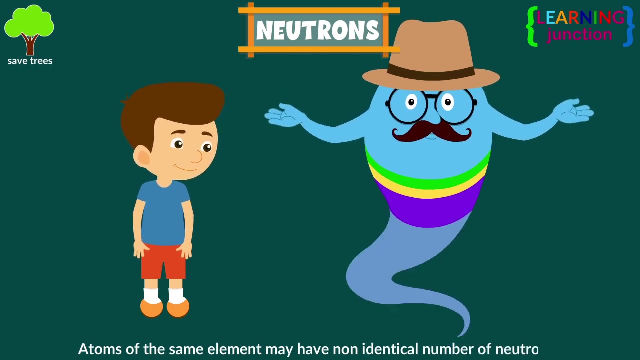 with no electric charge and a mass slightly larger than that of a proton. It was discovered by a British physicist named James Chadwick. Protons and the neutrons combined make up the mass of an atom. Atoms of the same element may have non-identical number of neutrons. 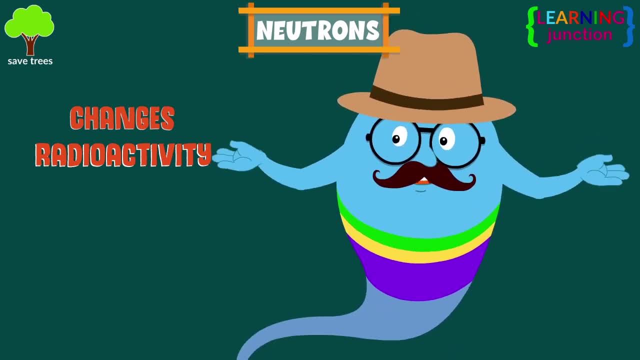 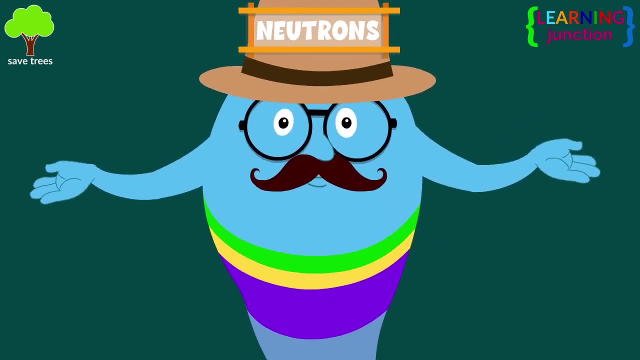 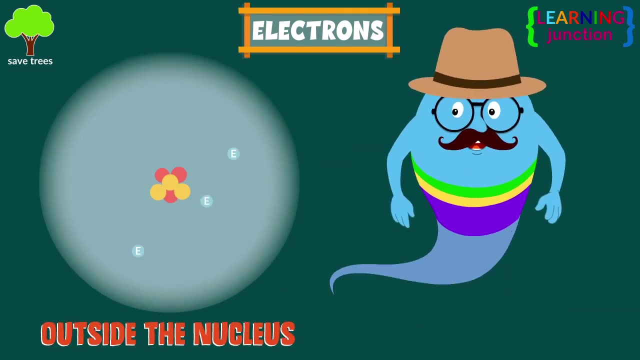 Adding neutrons changes the range of neutrons. The neutrons are the radioactivity of the particular element, without changing the charge of the atom. This is very important in nuclear physics. Now the electrons. An electron is a negatively charged part of the atom found outside the nucleus. 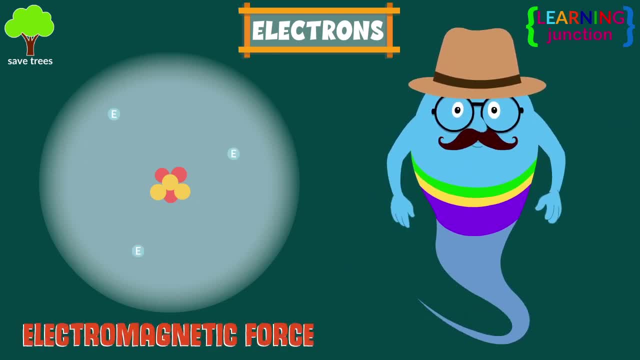 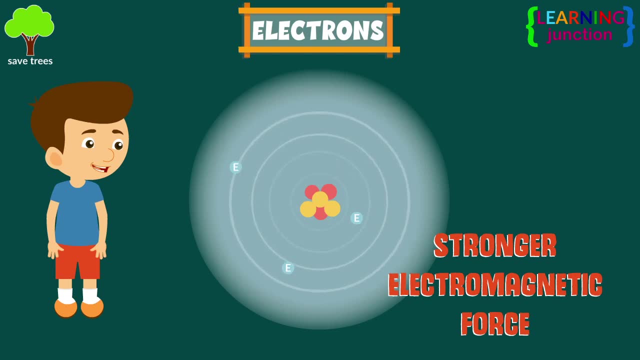 They are attached to the protons in the atom with electromagnetic force. The closer the electron to the nucleus, the stronger the electromagnetic force between them. Electrons can be found anywhere in the atom. Electrons can be found anywhere in the atom. Electrons can be found anywhere in the atom. 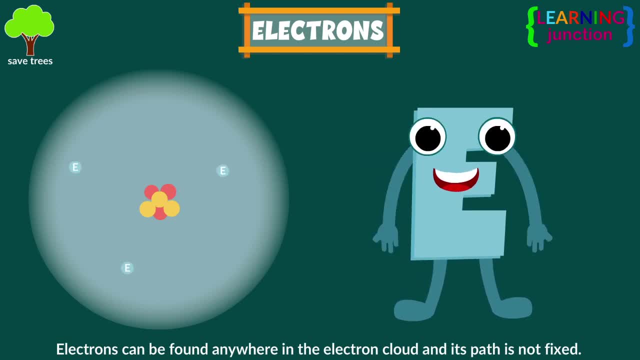 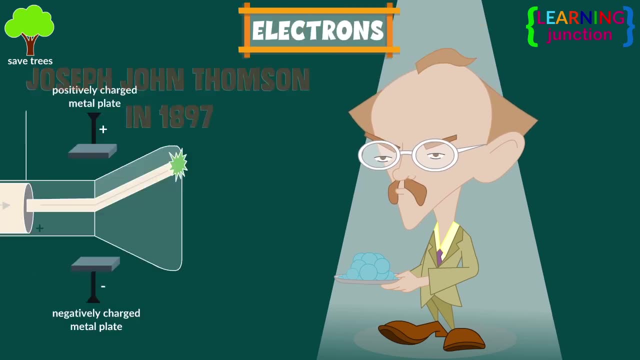 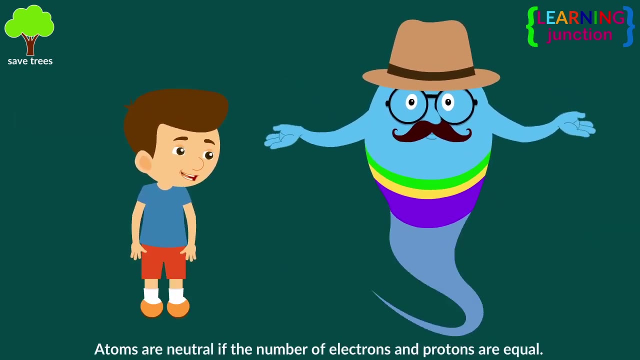 Electrons can be found anywhere in the electron cloud and its path is not fixed. Electrons were discovered by a British physicist, Joseph John Thomson, in 1897, when he was studying the properties of cathode rays. Atoms are neutral if the number of electrons and protons are equal. 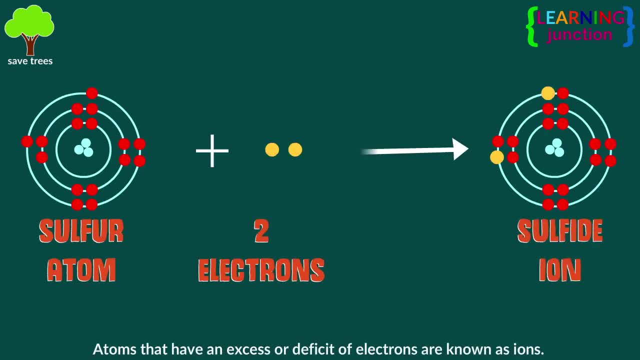 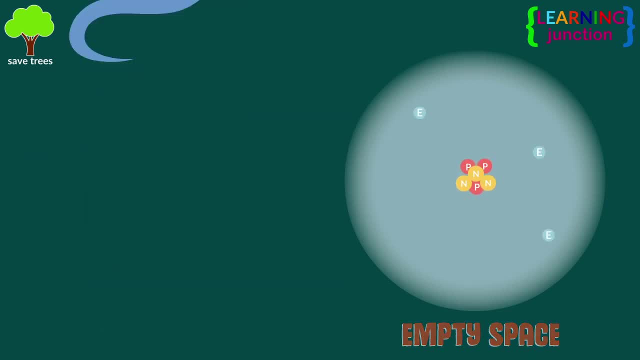 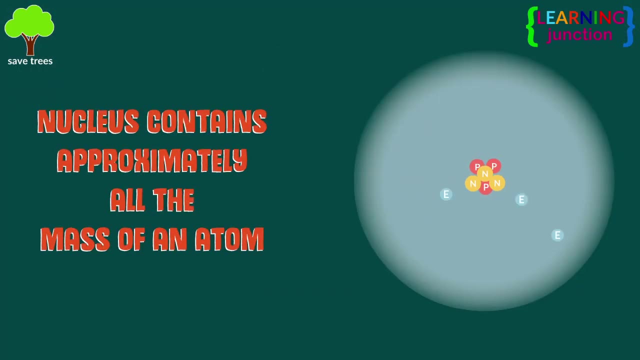 Atoms that have an excess or deficit of electrons are known as ions. The modern model of the atom shows an atom that has mostly empty empty space. In the center is a small nucleus made of neutrons and protons. The nucleus contains approximately all the mass of an atom. 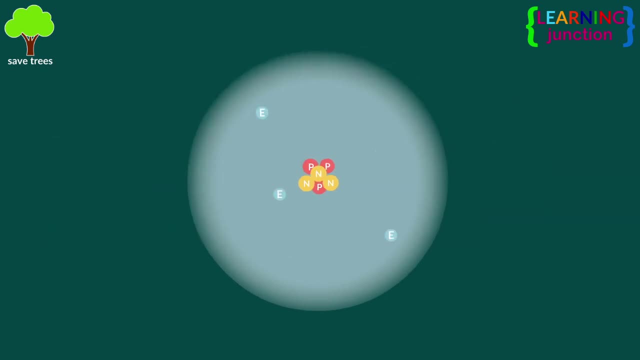 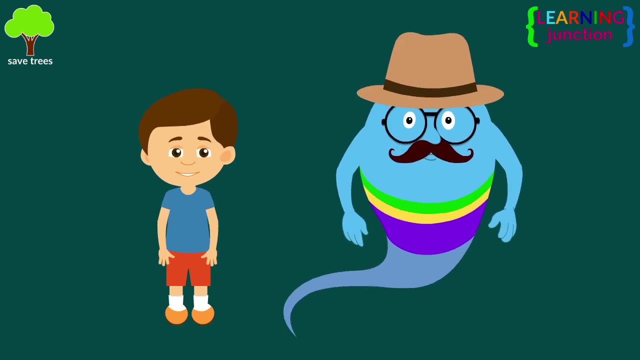 Surrounding the nucleus is a cloud-like region, with electrons moving too fast and too unpredictably for you to know their exact location. Now you know a lot about atoms. Stay tuned for more videos. Bye-bye. 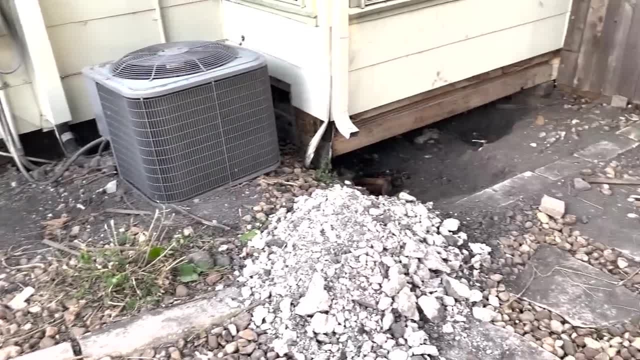 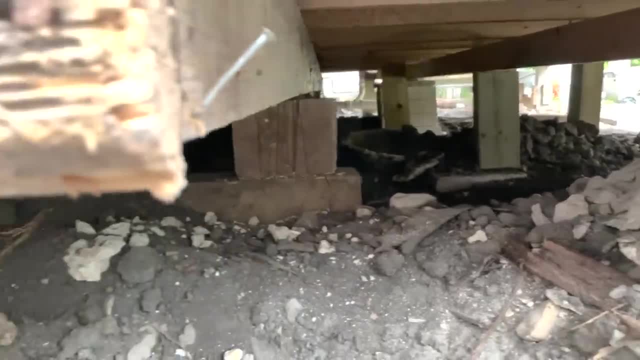 When we bought our house several years ago, we fell in love with every part of it except one: the foundation. At 75 years old we knew these old piers were just about finished holding this old house up. This year we finally bit the bullet to have them replaced. Any homeowner. 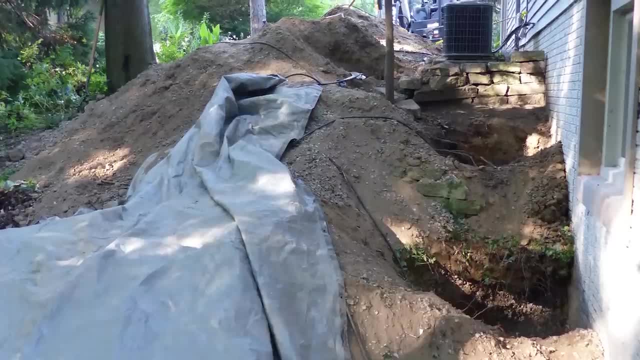 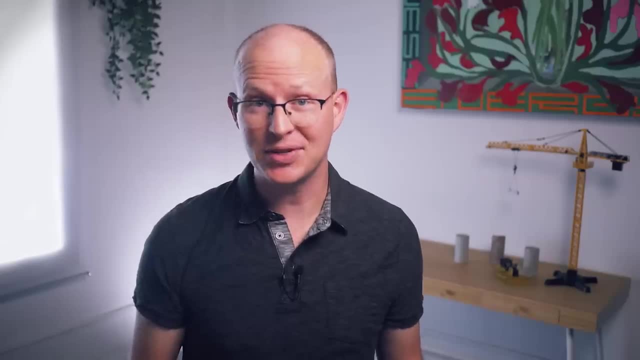 who's had foundation work done can commiserate with us on the cost and disruption of a project like this. But homes aren't the only structures with foundations. It is both a gravitational necessity and a source of job stability to structural and geotechnical engineers. 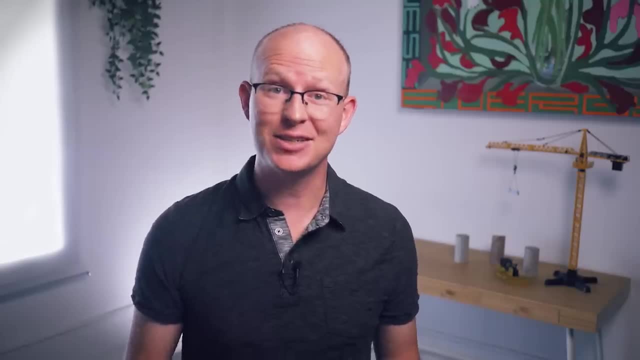 that all construction, great and small, sits upon the ground, And the ways in which we accomplish such a seemingly unexceptional feat are full of fascinating and unexpected details. I'm Grady, and this is Practical Engineering. In today's episode, we're talking about foundations. 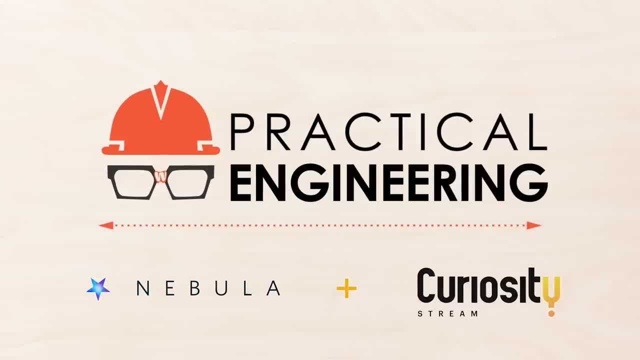 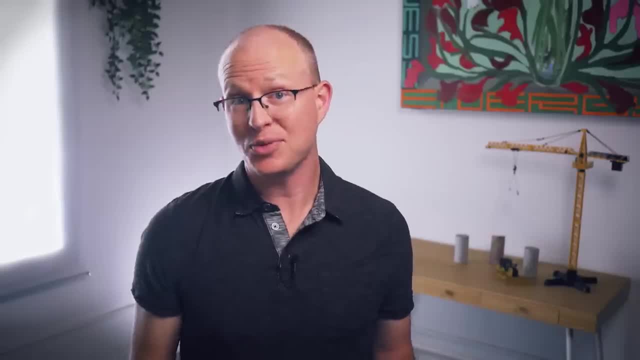 This video is sponsored by CuriosityStream and Nebula. More on them later. There's really just one rule for structural and geotechnical engineers designing foundations: When you put something on the ground, it should not move. That seems like a pretty straightforward. 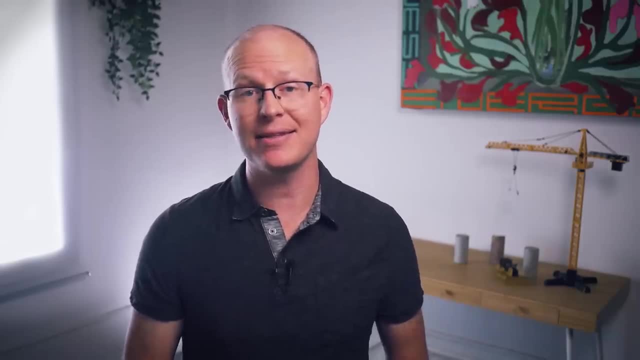 directive. You can put a lot of stuff on the ground and have it stay there. For example, several years ago, I optimistically stacked these pavers behind my shed with the false hope that I would use them to build a house. I didn't know how to do it. I didn't know how to do it. I didn't.